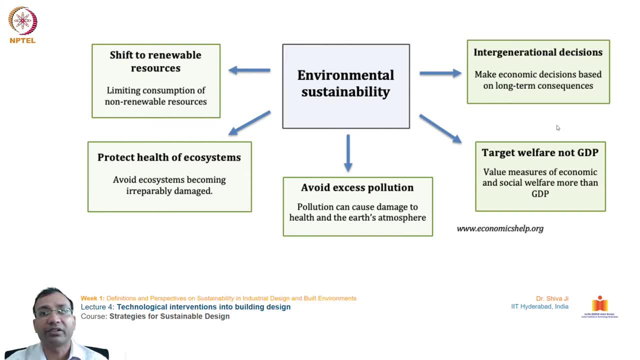 to the normal which was there in the pre-industrialized world. The second part: target welfare, not the GDP. Well, it is very important as we were discussing like how the humanity should be, like taken care of, how the society should function. 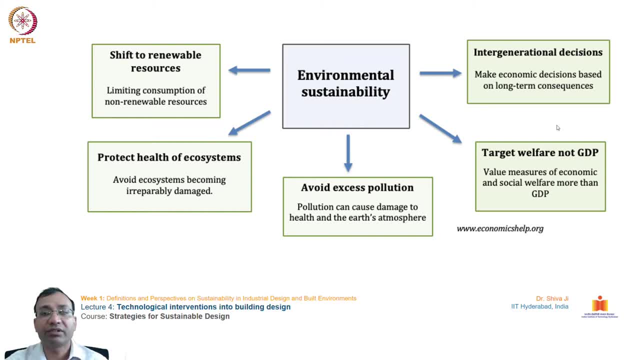 how the like, equity, cohesion and the value system actually works. So always like a development cannot be measured in terms of like GDP or the gross domestic product. So economic, like parameters. wise countries actually have this actually system in place today to measure the development of that. 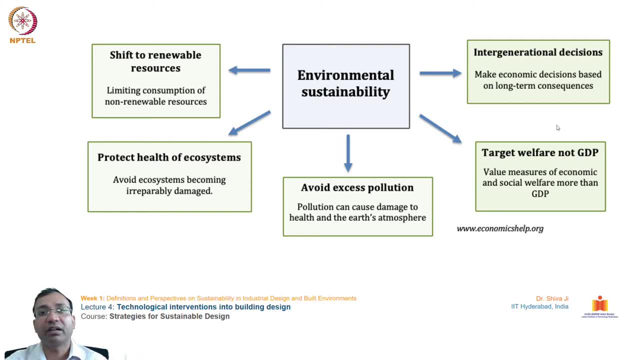 country in GDP terms, But GDP is not enough to assess a one person's actually well-being and happiness and how well he is able to live his life. GDP is not actually overall, cannot be an overall indicator of the success of any like a country. 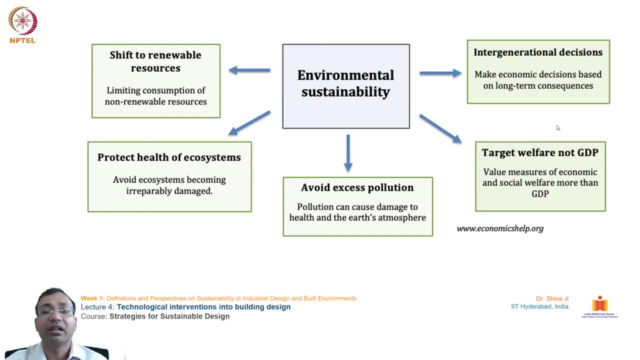 So the value measures of like economic and social welfare I have. actually they carry more value than the GDP only. The third one: avoid excess population. Well, population can cause to the damage to the like a human body and the environment and the overall ecosystem It has. the 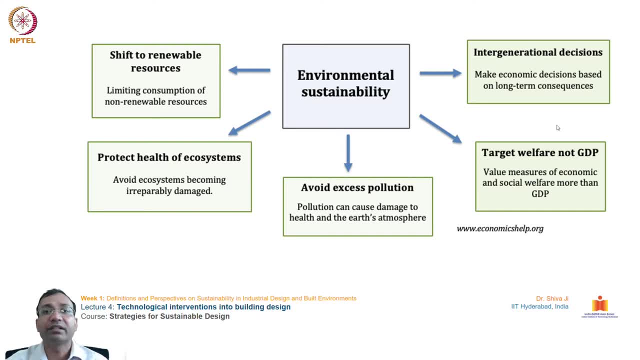 potential to actually disturb the ecological balance. So the pollution actually should be taken care of by each and every means, Because whenever we are like doing any like industrial, like procedures or manufacturing, or even like we are trying to provide some services, for example like aviation, So in turn of like 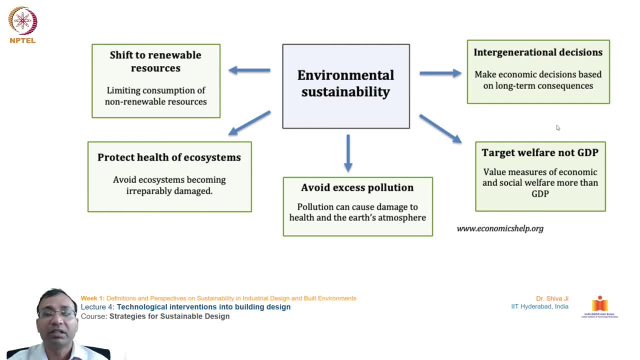 doing so. there is a lot of like a pollution happening in all of the like sectors like air, water, earth, soil, light, noises. There are several actually types of pollution, even radiation pollution, radiation and so on. So the question is, how do you manage it? 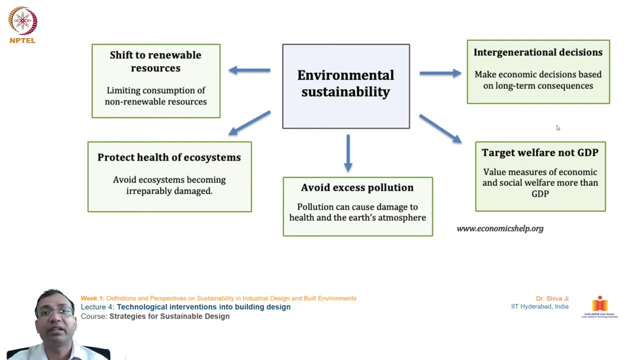 So the question is: how do you manage it? So in a way, it is actually a little bit like the nuclear reactor or so like one of the most considered to be one of the very like environmentally disastrous ones, Because in case of like any like such eventuality or accident, 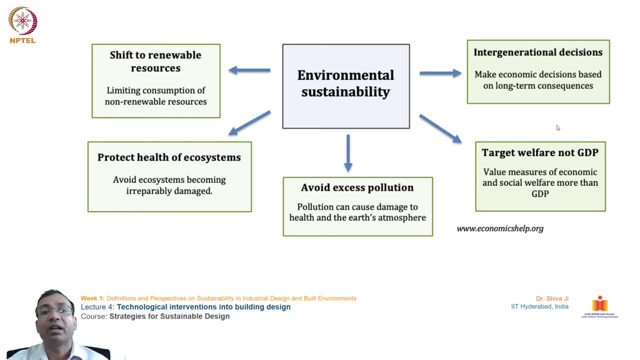 the catastrophic actually resultants will be very big, Like we are all aware of, the world's first like a nuclear disaster took place in the Chernobyl, Russia, And the Chernobyl is a place where it is, like I said, that it cannot be habitable for next like a thousands of years. So that place, 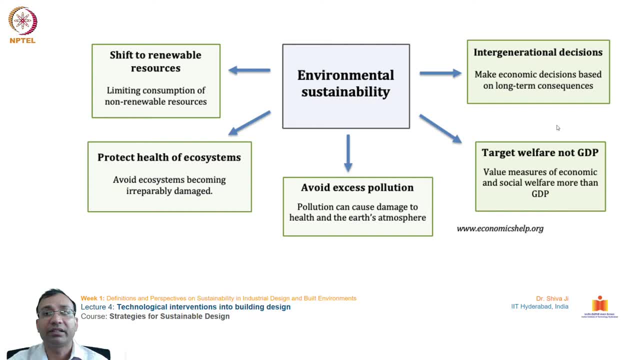 so that place is so contaminated with the high level of radiation that is, it is not safe for the like a human. so, like the second, actually accident happened in the fukushima, japan, where the nuclear reactor got actually burst for some regions, and then in the in the coming like a. 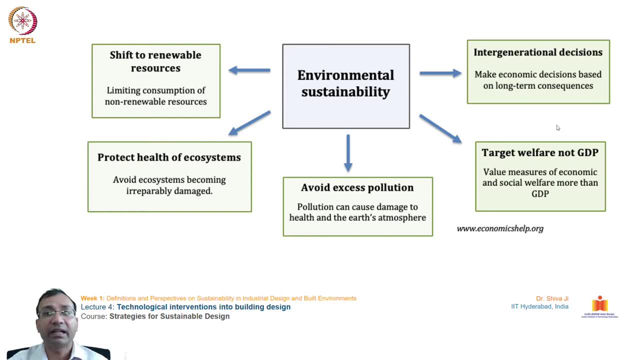 month there was this tsunami and a lot of like rain and that actually took away some of the- you know- parts of that, some of the radioactive material with it in the ocean and in the nearby area. then it was observed that radioactive material was found till like a very farther. 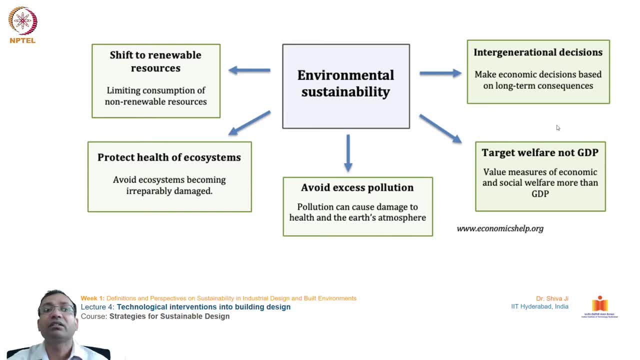 distances from the place of like fukushima. so nuclear, actually, reactors have this very hazardous, like a very high hazardous quotient, uh, though they are the source of like a very high volume of energy by putting a very little of like a material, but the toxicity and the radioactive. 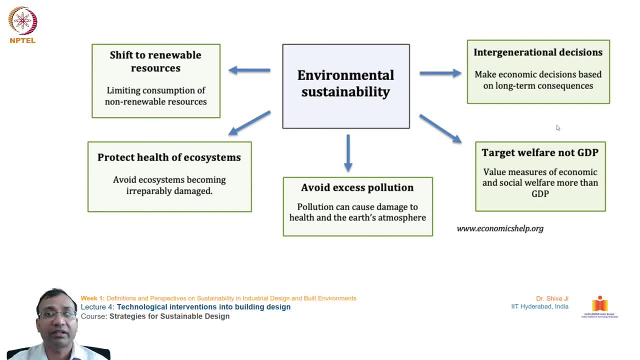 material and radioactive quotient and this overall like a pollution factor is very high with them. so we must take care of like each and every types of like a material or pollutions which are possible with the manufacturing of any of these like a light industries. and the next one says about 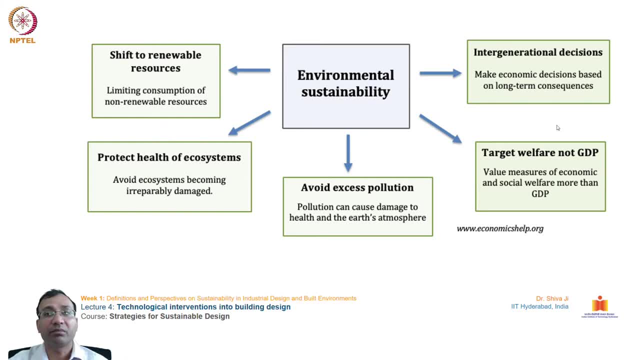 protect health of the ecosystem. well, the health of the ecosystem is very important because if the balance is now is gone, then there will be a lot of like repercussions and that will become like a irreversible, actually position, from the point where the balance of the earth cannot actually come back. 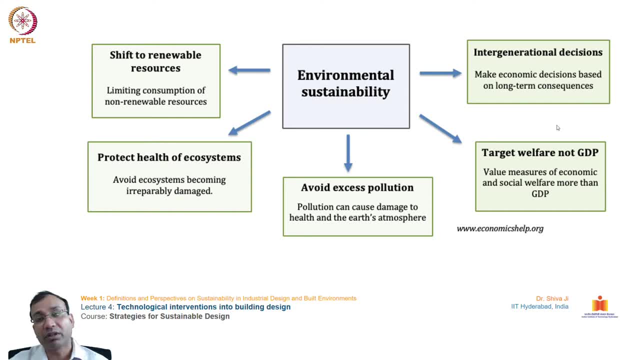 to its normal position. and the last one shift to renewable resources. well, uh, we have been discussing, uh, resources are like a finite, finitely available, they are not infinite. so the supply- and you know there is a supply of these materials for, like, our consumption- is very, very limited. 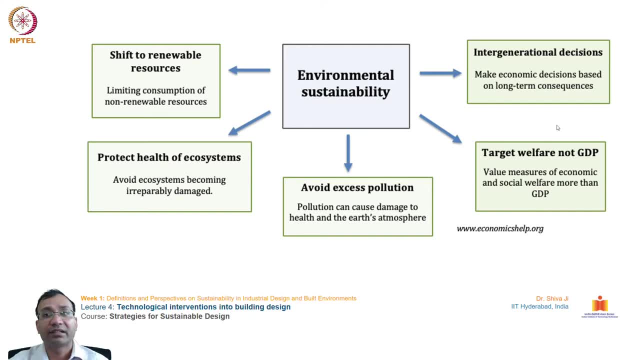 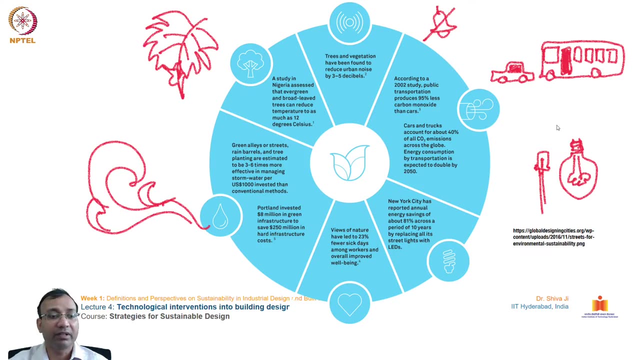 so we must consume them in such a way so that nature gets time to heal itself, gets time to like, restore itself, gets time to bring it itself to the balanced position. these are actually major principles around environmental sustainability. we will move ahead from this and we will see uh some, uh some discussions. so a study in nigeria: assist that. 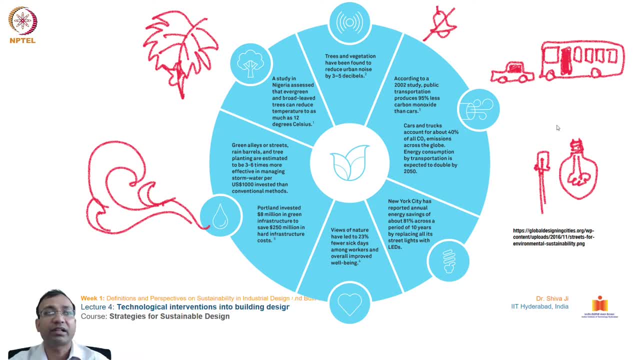 evergreen and broadleaf trees can reduce temperature to as much as like. well, i think it is very evident. we may have noticed whenever we enter to like a foresty area or maybe even cantonment areas of our like major cities in india, okay, or even like a bigger institutions who have 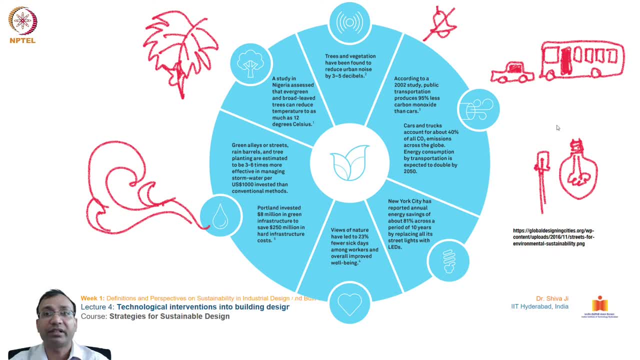 bigger green campuses, okay, for example, like some universities and some institutions. so we observe actually a significant drop in the like a temperature the moment we enter into those areas. so why is so? so it is because of the, the dense vegetation, the dense plantation which is there in those uh area. so because of uh, actually, that the temperature, the ambient temperature of 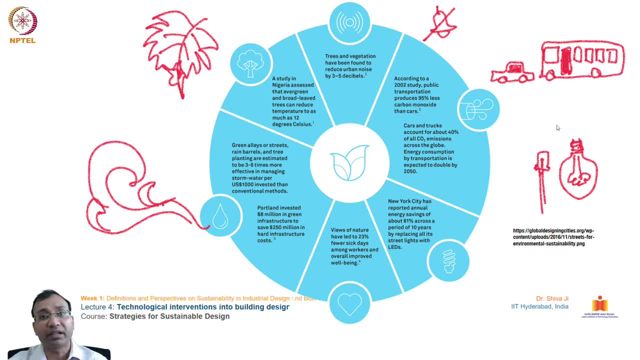 that area actually remains slightly lower than the main, actually the business, uh like, uh, parts of the like, a business district, part of the city. so this actually observation is based off of, like a recent observation based out of like a nice area. the next one, the green alleys or streets. 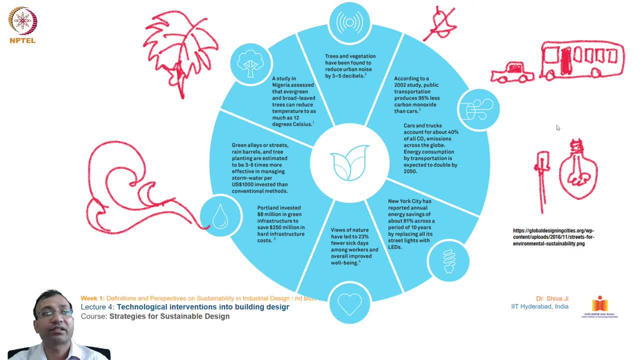 rain barrels and tree planting are estimated to be three to six times more effective in managing storm water. per us dollar, one thousand investor net conversion methods. well, we have been knowing the traditional, like water sheds and uh, these are like a rainwater, like a management, it happens to. 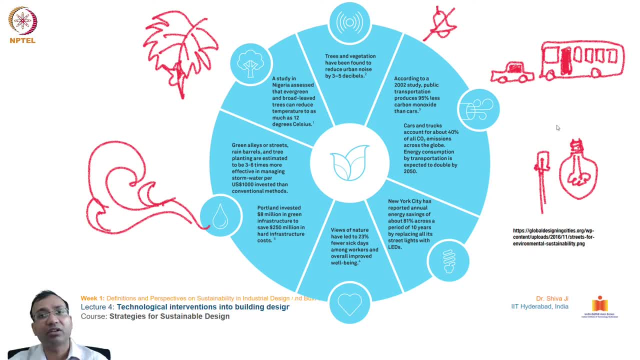 the trees. so why forests are important? not just for the like vegetation and oxygen, they actually we play a very important part in managing, you know, water. so whenever the forest or the green areas, they uh, actually receive the rain water, they hold actually a large amount of their own that rain. 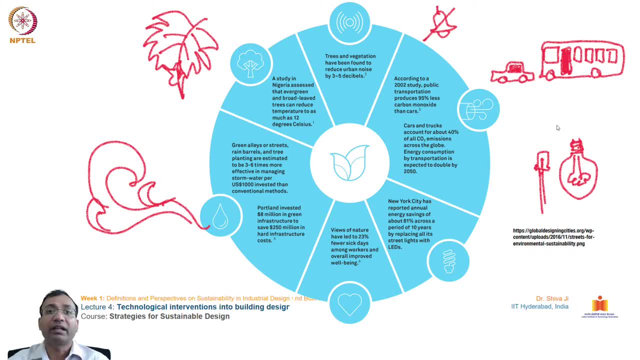 water in their roots, in the top soil, okay, and that water remains and gets filtered over the time and it starts like a coming down through, like a smaller, like streams, and in the form of the rain water, and that is how actually rivers also get born, because from the mountainous regions 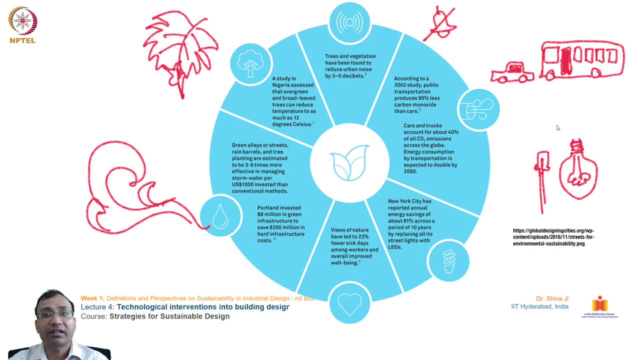 from the like a green area areas, this water actually starts seeping slowly, slowly. if there is like a barren flat surface, all of that rain water is going to run off in like a one stream and then and then the next time there won't be any water left behind. so that is not good for the 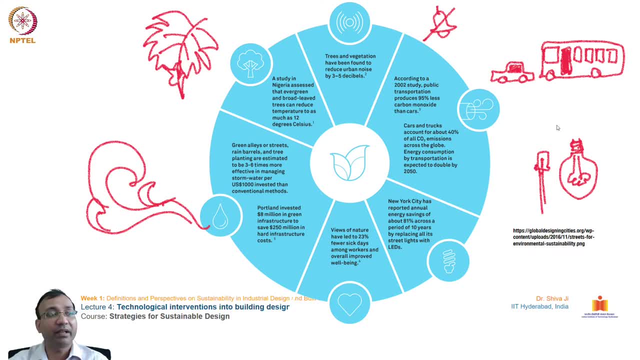 actually ecological balance. so this trees actually play a very important role. uh, if we try, uh, or retaining this water through like a conventional means, like a other conventional means, like a dams and all that, so that can retain the water, but not in that actually quantity and plus the creating dams and like such structures have their own ecological actually impacts on the. 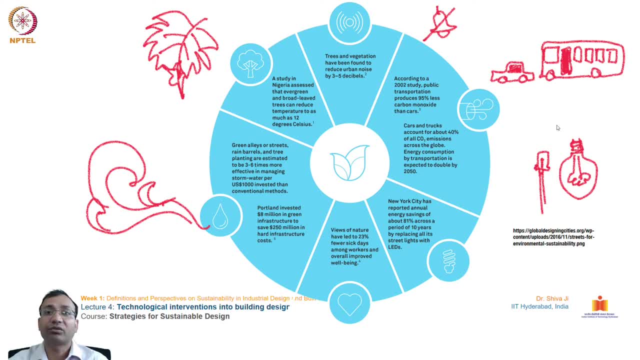 like a place, so we should avoid as much as possible, and so we should always like increase the number of plantation, the density of plantation, vegetation in the like a greener areas, and the next example related to this is the. uh yes, we have planned and invested eight million dollars in green. 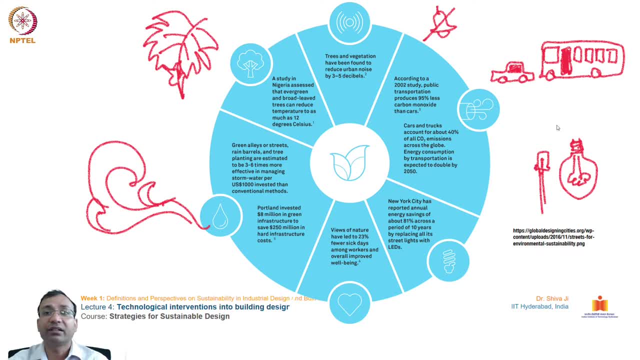 infrastructure to save 200 million dollars in hard infrastructure costs. well, that's an example where these uh softer investments into like a nature always pay like a much yield in terms of like the solid hardcore, like infrastructure, like activities, for example, like if you want to establish like a a greener areas, if you want to have like a fresh air for the supply, if you want. 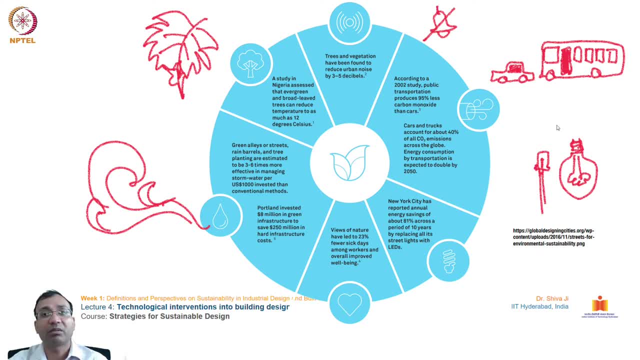 the. if you want to have like a continuous green running system, then that means you should try to find a new area to build stop and perennial water supply for the cities and urban settlements. So we must actually go for the natural means of managing these resources in place of managing them actually through 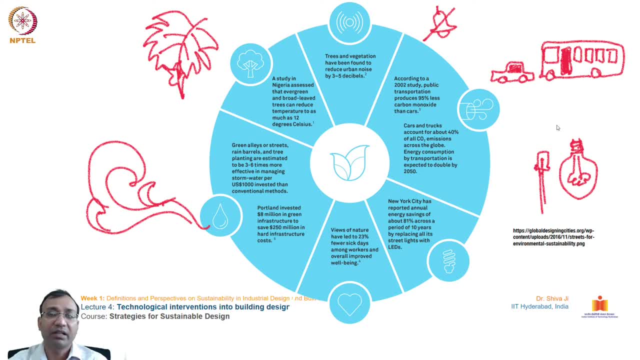 constructed means or hardcore infrastructure generation, Because they can do that job but they will take a lot of money plus their repercussion. But natural means they do not have any such repercussions. Natural means actually help the nature to regenerate and grow back. So it helps actually even other species and other living beings to 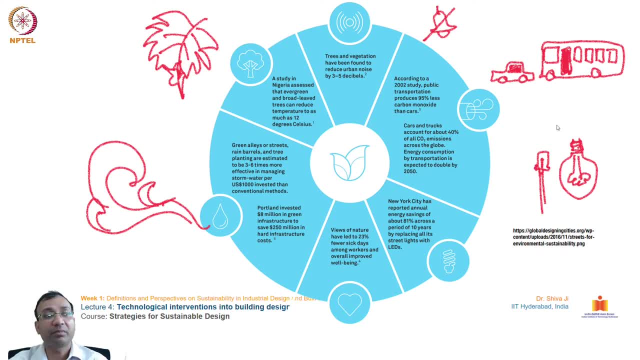 come back to their normalcy. The next example says: view of nature have led to 23% fewer writings among workers and overall typical of abused another. Well, this has a lot to do with the psychological, actually, feelings of our- seem Voilà, the humans We as, like a. 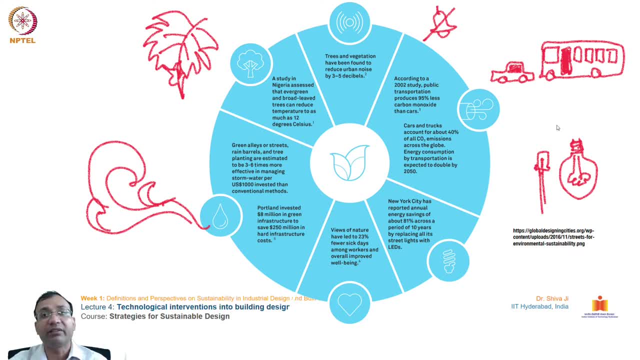 social being. we, as a human being, we always feel elated and we feel free, we feel like a good in an era, natural, surrounding where at least we can see, we can observe, like some scenic things, we can see other, like a human beings, like, uh, doing their activities and normal, choosing compared to like. 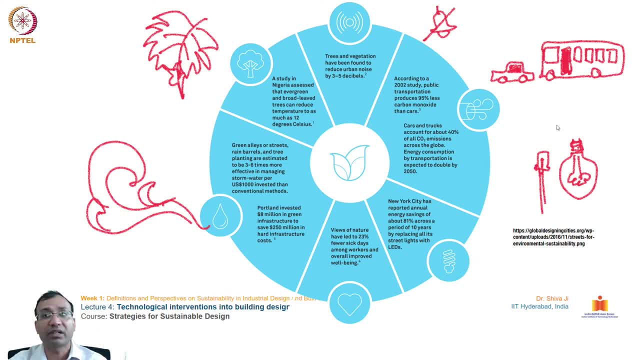 someone sitting inside a closed actually environment, closed atmosphere, where he cannot, he or she cannot even see outside. so there are always like a such psychological actually impacts of like a such like about places. so it is always like uh suggested to have uh to deliver, to give actually as much view as possible for the workers from their offices or from workplaces so that they 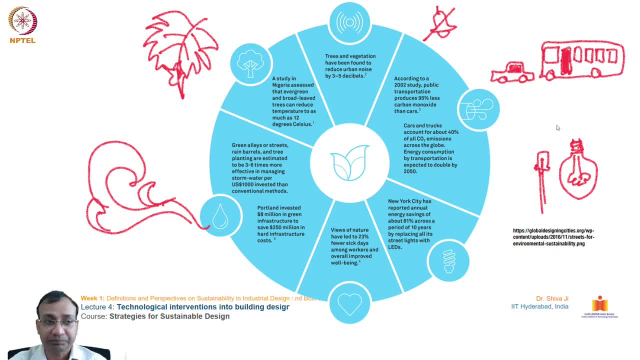 can keep themselves like psychologically connected to the outside world. the next example says new york city has reported annual energy savings of about 81 percent across a period of 10 years by replacing all its street lights with x. well, of course it's a proven fact, i think, from from everywhere. 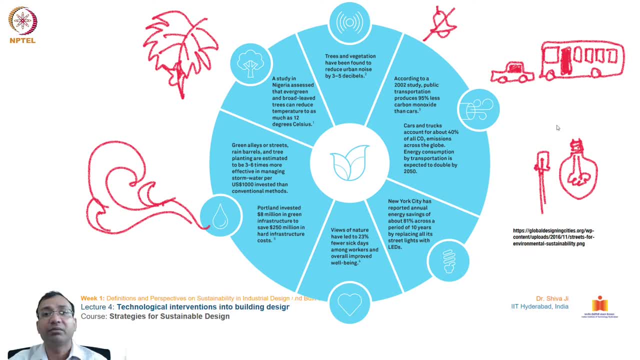 recently, i think in the last few, like last one decade, there has been a significant push from the government of india and the state governments also to replace those incandescent bulbs with the lcd or led based bulbs. so these uh, actually electrical devices have been highly subsidized also and they have been given to like each and. 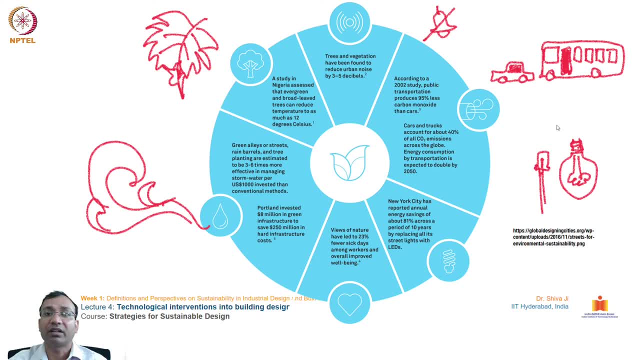 every household on the through the like a medium of this rationing on a like a subsidized rate, so that they can replace those uh power hungry, actually uh lamps with these power savings. so it's not just new york, i think it is true, for like every place so, and such actually efforts are. 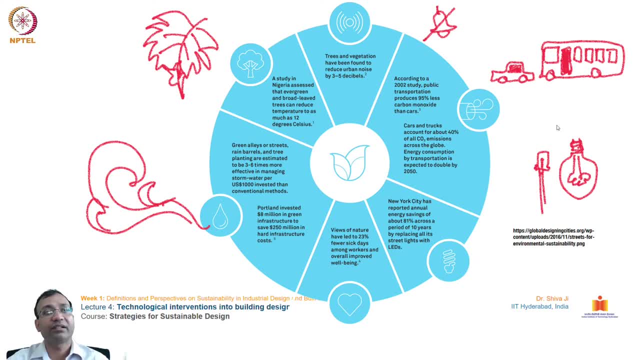 being done for the society. the next observation says cars and trucks account for about 40 percent of all co2 emissions across the globe. energy consumption by transportation is expected to double by 2050.. so here we can see these uh traffic based like these are transportation based. 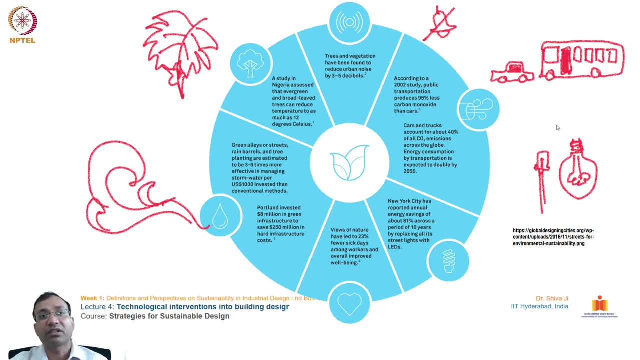 actually, uh, these exhaustion and then the missions, they have caused actually a significant, uh, actually, contribution to the ghg emission, majorly the co2 and well. so, and if you, if you compare, like, uh, the number of occupants who can travel in a car and number of occupants who can travel in a bus, so obviously there is a stark difference. so why not to save on these like an individual, like personal vehicles, and go for, like you know, mass vehicles or the public vehicles? according to 2002 study, uh, public transportation produces 95 percent less carbon monoxide than cars. well, obviously, the fact i was like a stating just right now: uh, the, the public's, uh. 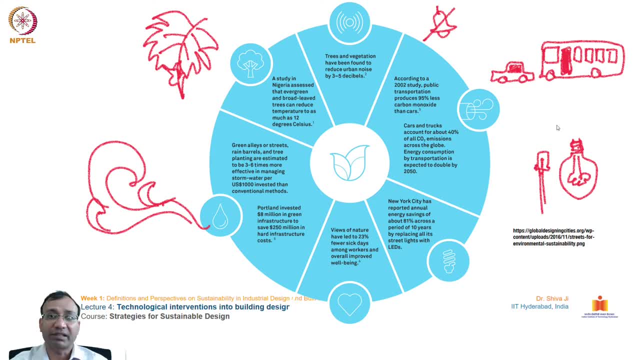 actually transportation medium, of course, will save on the numbers. okay, for a set of like around 40 people, one bus would be enough. for a set of like a 40 people, we at least, at least, need like 10 cars. so, if we go by that ratio, the number, the amount of emission which will, uh, be exhausted from the 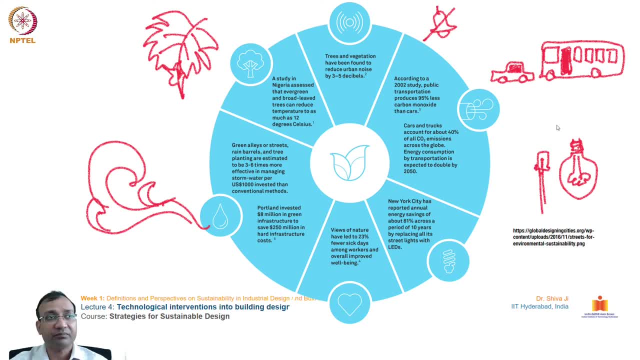 like a public community will considerably be lower. and the last one says trees and vegetation have been found to reduce urban noise by three to five decibels. well, it is true, uh, for the like a temperature drop, as well as for the noise reduction also, because, uh, vegetation is a one very good. 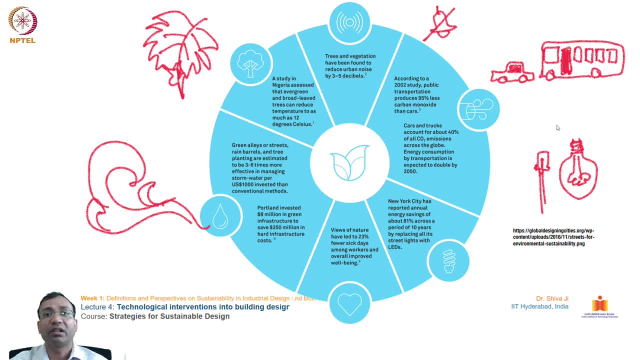 source of actually noise absorption. so it works for like absorbing the noise, whether it is for like a traffic from like any some manufacturing or some machining plant, you know, or any like such a noise producing actually uh, entity. so a dense vegetation helps always for the sound as well as. 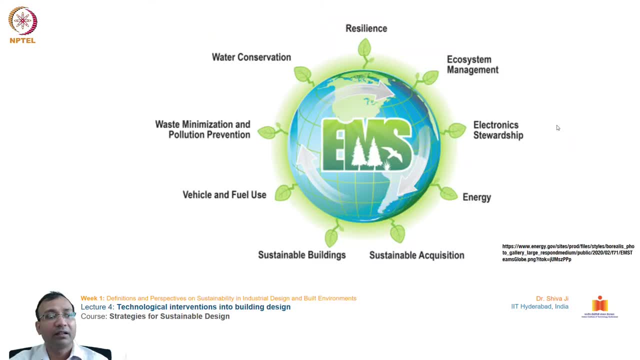 reduction. uh, what are the actually major features of uh this? environmental, like a sustainability, so the capacity to have like this resilience. what is resilience? resilience is a capacity to come back to the normal position without much of like external intervention. so it is like an inherent quality. it is the inherent actually property between uh in the system. 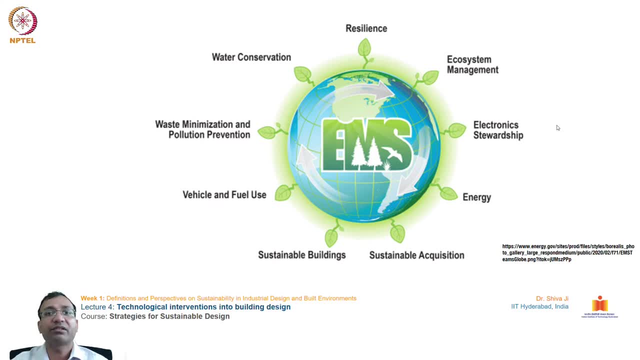 which, which, which, which tries to you know, uplift that system once it has gone through. one is one's has experienced some catastrophic event or some some kind of like damage, so that capacity is known, known as like resilience. so a resilience is there in the nature by default, like, for example, 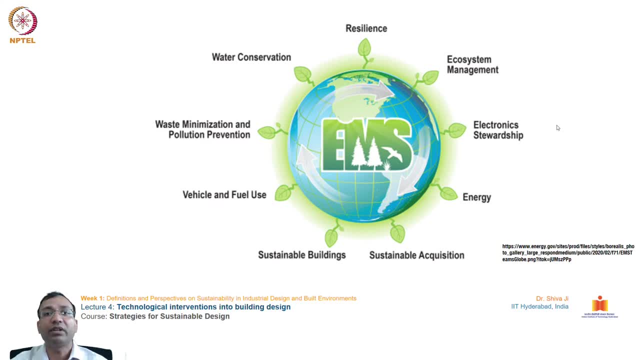 like rivers, so rivers have their own like a capacity to heal themselves. if there is some like a kind of pollution or some some toxic material which is thrown in the river, the river or that water body, whether it is a lake or something, it takes some time and 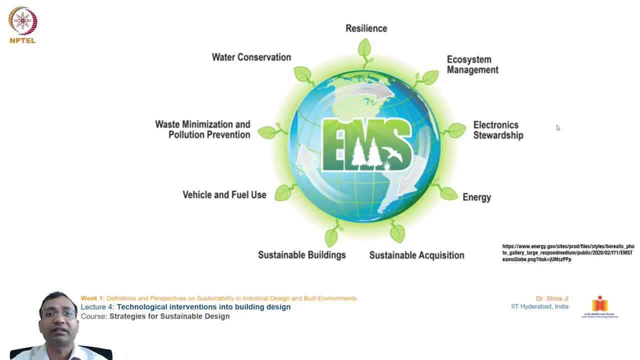 rejuvenates from that. so that is a resilient actually capacity of that thing. well, the overall, like a planet itself, if we see from the like environmental perspective, has some resilience to come back to, like a normalcy, to restore its normalcy, but of course it has some threshold. it. 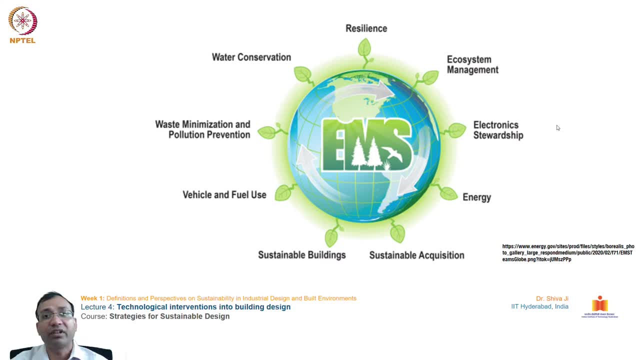 has a critical, actually uh, value after which it will become very difficult- and there is some value after which it will become kind of irreversible- to go back to the normal one. so we must actually take care of this, uh, the, the bio capacity, or that resilient actually capacity of the ecosystem. 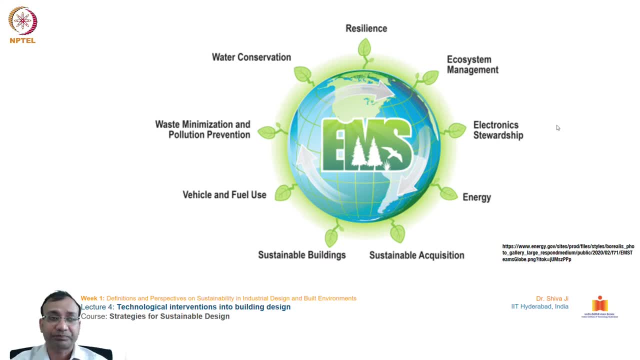 so that it it enables itself to restore. and then there is a eco management system so we can like a manage, like an ecosystem in such a way that it sustains for a longer time. then there are like a lot electronic stewardship, energy sustainable acquisition, sustainable buildings, vehicle and fuel. 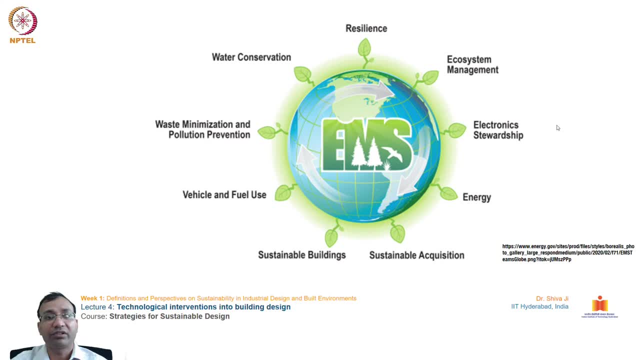 use, waste minimization, pollution prevention and water conservation. these are the one- actually few few of the major actually activities around environmental sustainability which play actually a vital role and they form actually the major component within the environmental sustainability, like energy we have been discussing, buildings are the majorly. 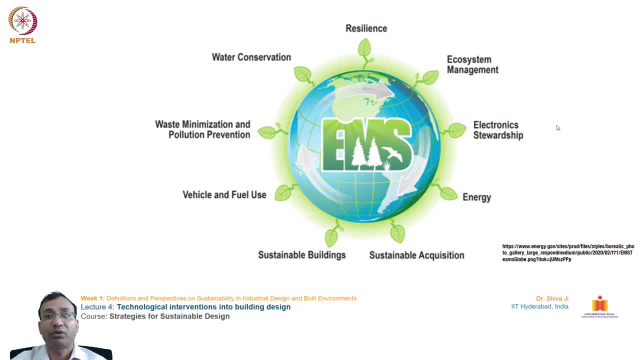 responsible for the uh consumption of around up to like a 40 percent of the total world energy produced. that's a huge amount. it's even more than the industry sector. so if you see like buildings are the single largest consumer of the total energy produced in this world, okay, so even if 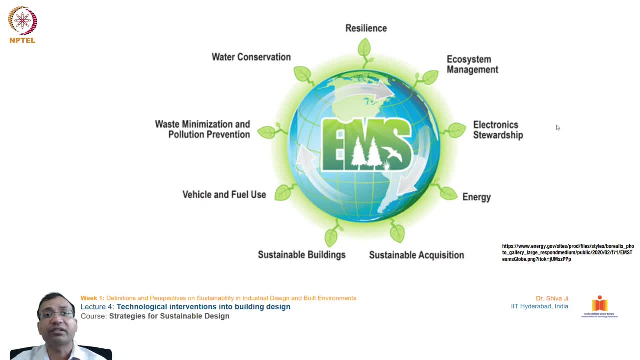 there is a like, an improvement of in like, in the fractions, okay, in the, in the scale of like this whole world, that the overall volume will be extremely high. so even if there is a saving, saving of saving of a very small like, a fraction or small percentage, 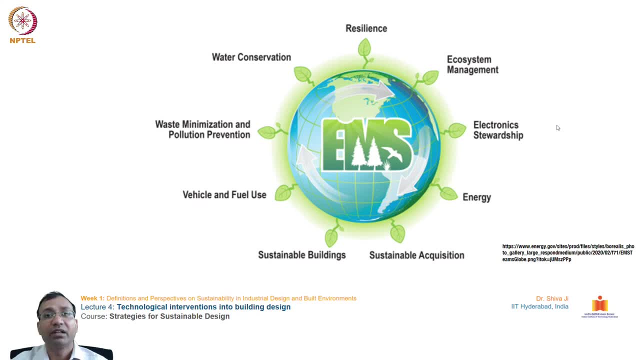 the overall saving will be very high. so we must put our efforts to improve actually this situation. and sustainable acquisition actually talks about uh sourcing materials in a responsible way, sourcing uh like, like, for example, uh trees. so why can't there be a crop cycle for like a? 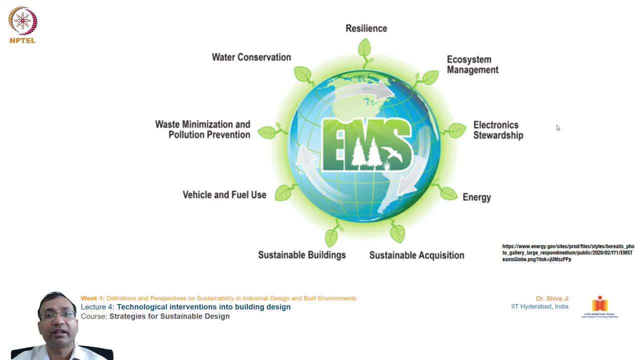 harvesting of trees. well, some countries like canada and new zealand- they have already uh have such systems in place, so they actually have some managed forest from where actually they do like a annual cycles of a forestation and they cut those trees for like a uses and 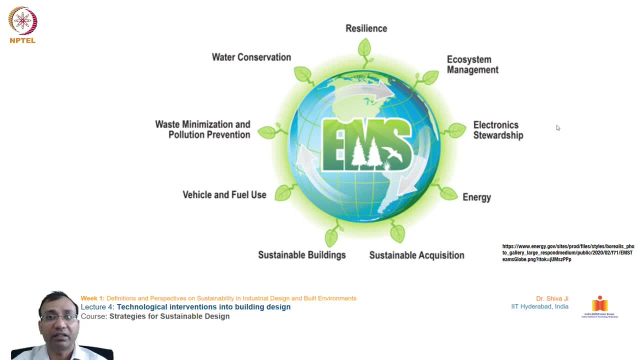 consumption at the like, a cycle of the, that, that that those trees specifically, and uh, every year, if you point, plant like x, area of, like a land with the trees. so after that, in number of years, we will start getting those x, uh, like a, like a area, will start producing those. 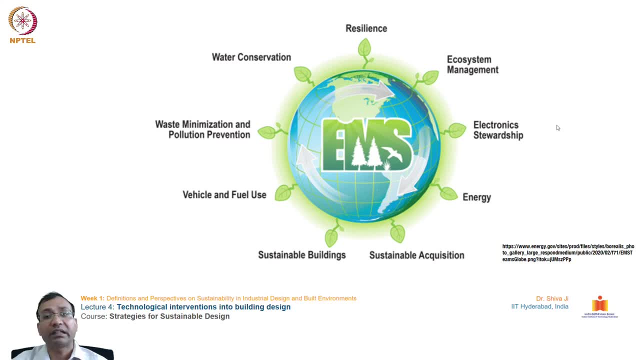 number of trees and there is still no- uh, practically, uh, completely replaceable, you know, alternative material available for, like a natural wood or timber. so why not to have to start having actually such procedure to have forest as a like a cycle of crop? and well, of course, there is a like, a point of 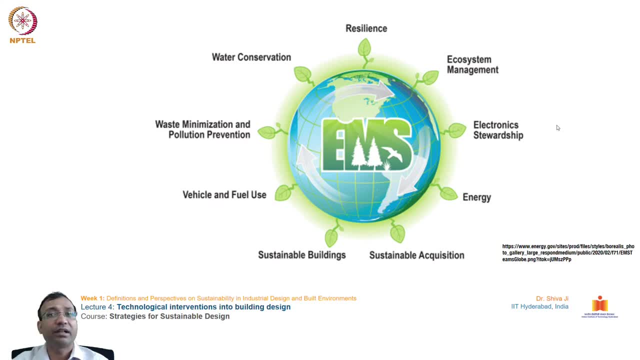 vehicle use and uh fuel use. so, as we saw, like, vehicles and such things are the single largest emitters of the like a pollution. so we must actually work to prevent uh these things, waste minimization and pollution prevention. so, of course, waste, uh like, uh with the like as a byproduct of most of 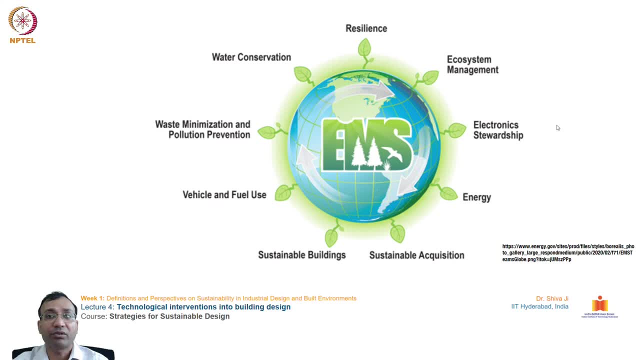 these industrial like processes. these days there is a huge amount of waste produced. so how this can be minimized? because nowadays landfills and these, uh, these things are becoming very common and uh, it is almost like a practical situation, a practical compulsion, that all of the waste which 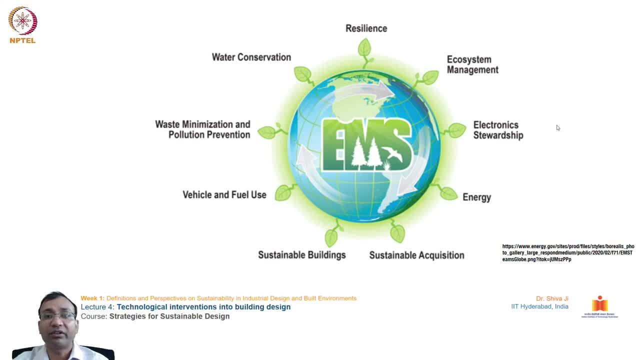 is being generated is not able to get recycled or treated properly, and it is landing into the landfills. okay and uh. most of the like indian cities, most of the world cities, are actually plagued by uh this situation, though there are some countries who are doing uh fairly well, like 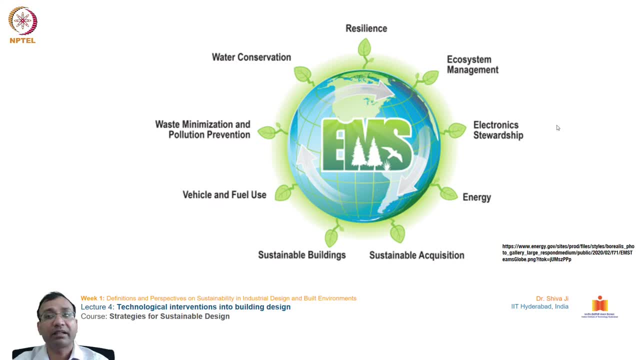 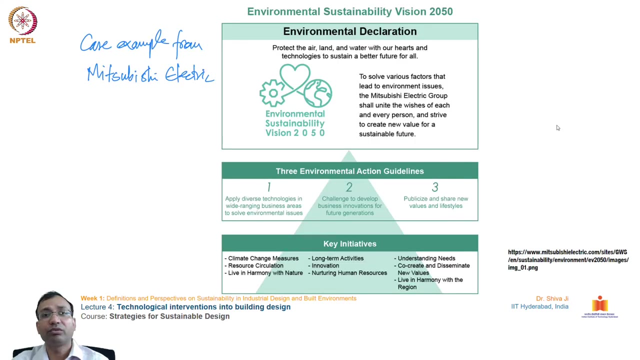 sweden and some countries. they have actually developed some mechanisms to go for like a power uh from the waste and they, they are actually running out of waste. so this is really strange and i think it's worth uh emulating in the uh in the elsewhere. so let's move on to like the next. 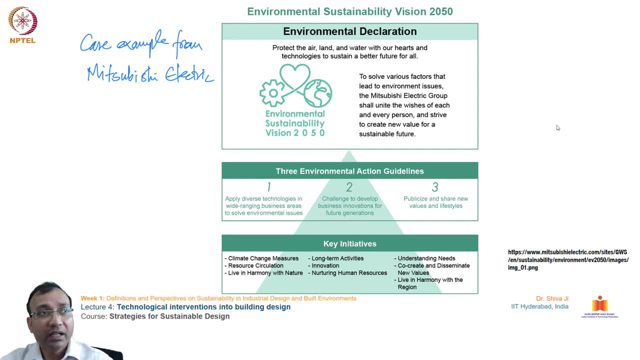 slide here. i have taken it from like a mitsubishi electric company which has actually taken up uh this cause as a, as a like a inspiration to drive their like uh manufacturing and other like things from their factory and they have, they have given actually declaration, they have actually set up some guidelines. for example, the first guideline says like apply 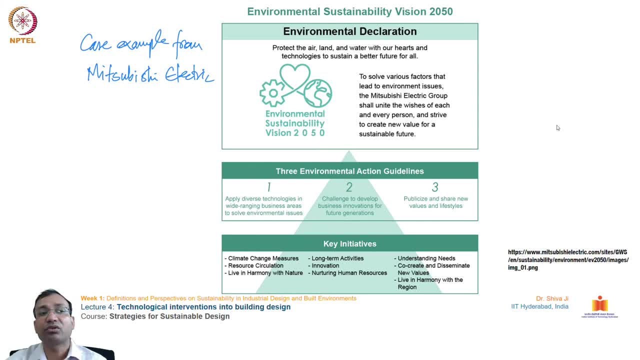 diverse technologies in wide-ranging business areas to solve environmental issues. so that means they are looking for some alternative technologies to deal with this situation. the second, actually guideline, says challenge to develop business innovations for future generations so that these, these innovative like ideas, innovative like business models, can help to sustain themselves. 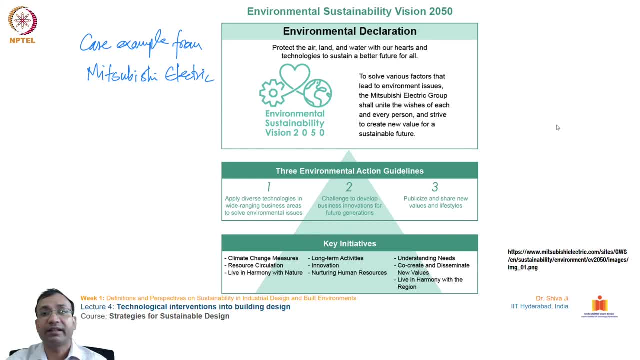 future generations also. the third one: publicize and share the values and lifestyles. so, like the new value systems, well, the uh and uh, these uh lifestyles should be like a you know, propagated in such a way which which can become a role model for the other, like other members of the society. 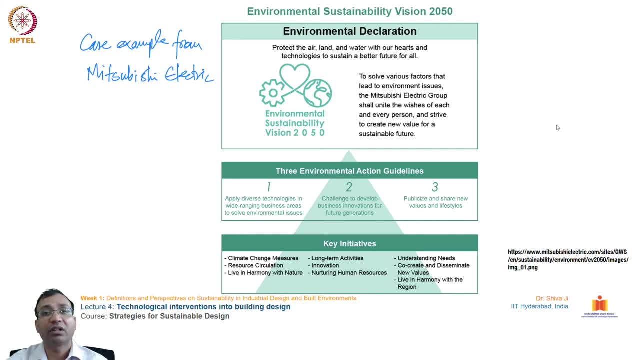 other members of the community. okay, those are like a which, uh, which, which are like a worth mentioning, worth actually emulating. so, the key initiatives: what, uh, this company has taken is the change measures, resource circulation, live in harmony with the nature, alarm long-term activities, innovation, nurturing human resources, understanding needs, co-create and disseminate new values. 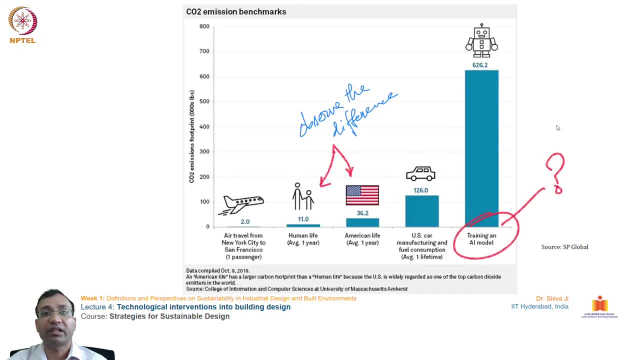 live in harmony in the region. so these are the actually key initiatives taken by this company. let's look at the co2 emission benchmarks of like a different, like a familiar things which we generally like come across so you can see on the on the x-axis, there are some examples. 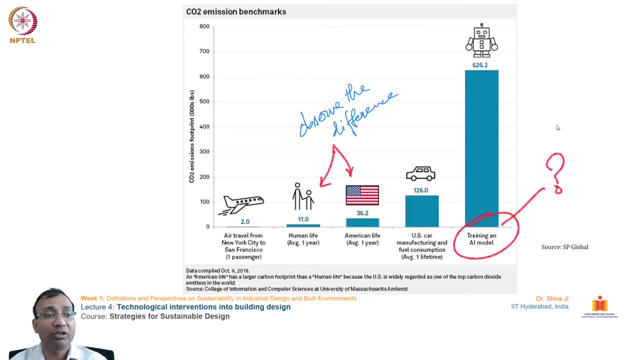 like air travel, one like a one year of like a normal human life and now one year of like an americans like a human life and the la. the fourth one says about uh the car emissions uh caused from like a one car in the us, and the last one says about like an ai model. so let's see on this y-axis. 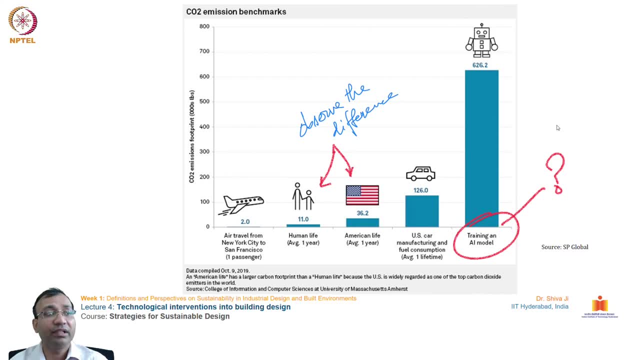 you can see co2 emission footprint. so here, like a, a travel from new york citizens to san francisco, uh, it, it emits around like two units, for example, of uh, the co2 submission. okay, so co2 emission of two units, uh, if you compare, like a one person's the one year of like a co2 emissions. so that is. 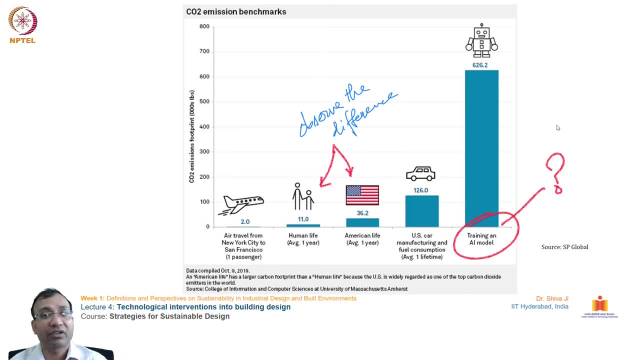 around 11 years, okay, and compared to one like a general human being from like an average, like a world citizen, okay. so the one single like american citizen himself or herself emits around 36.2 units than a normal like a human being which is a world citizen. so that means the per capita actually is. 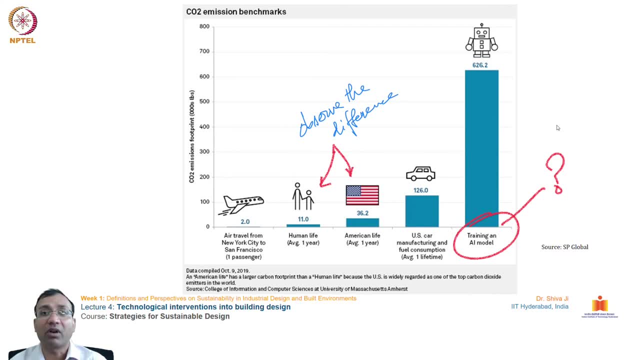 due to a mission of an american. okay, is three times the world average. okay, let's see, like a one year, one lifetime, like a mission of one us car is around 126 units, which is very high. and the strange actually entry into this table is this last one, training on an ai model. 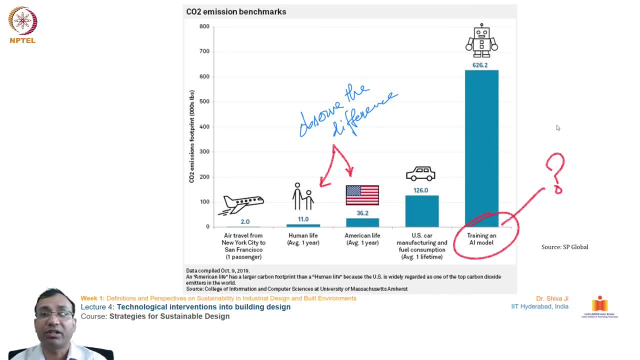 so training an ai model actually consumes 626.2 units of like this co2. compared to all other, this is very high, extremely high. so how this? even this kind of like a new technologies and these systems- uh are like a power hungry are going to have some. 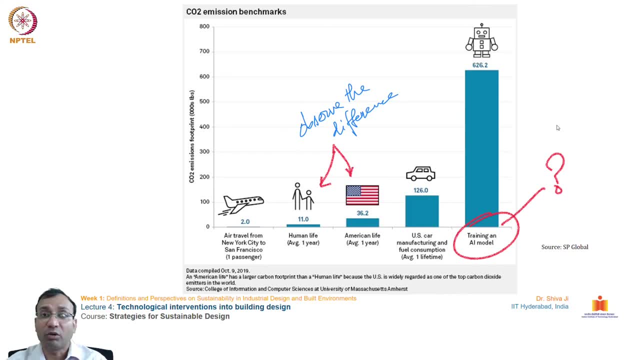 kind of impact. impact is actually eye opener actually. so we must actually go for, you know, analysis based observations only where we can conclude with the help of the numbers. otherwise sometimes most of our assumptions, uh, they sometime actually prove wrong. so we must actually rely on the calculations and the data in the next part of this. 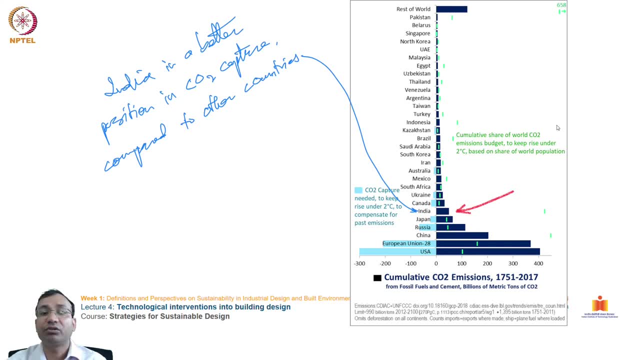 slide. so the data suggest over here the cumulative co2 emissions between the year of 1751 to 2017.. so from fossil fuels and cement, billions of metric tons of co2. that is actually uh unit what they have taken over here. so if you see the rest of the world, 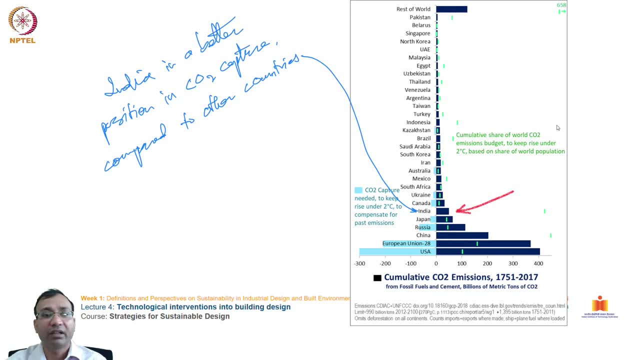 okay, emits around like a 140, 150, uh like a metric tons of co2, and usa emits a lone over 400 metric tons of ua2, has a has actually kind of excreted during this period, during this timeline. and the second comes, like the european union with the 28 countries and 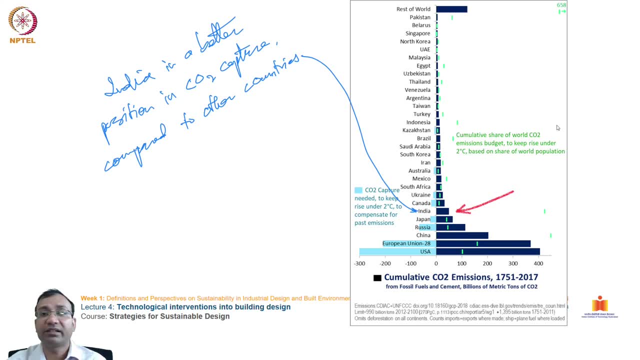 that the third one is the china. so china in the recent times has developed very fast and is developing very fast and is the one of the largest producers of the last largest and meters of the co2 also in the world. if you see the next country, russia, then japan and then comes the india. 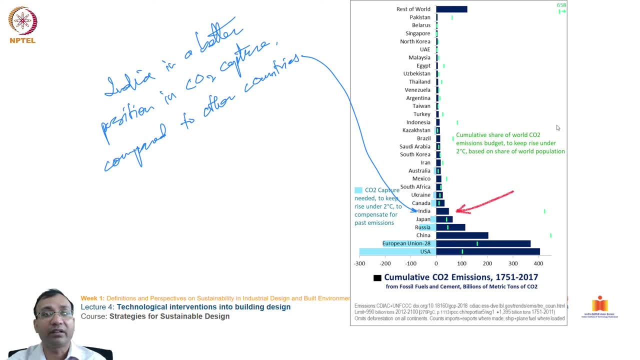 so the one uh amazing thing about uh india over here is, even if india is one of the uh big emitters- okay, it emits a roughly around like a 50, like a metric tons of, like a co2 it has emitted between this year, 1751 to 2017.. but co2, uh co2 capture, which is needed to compensate, actually, this. 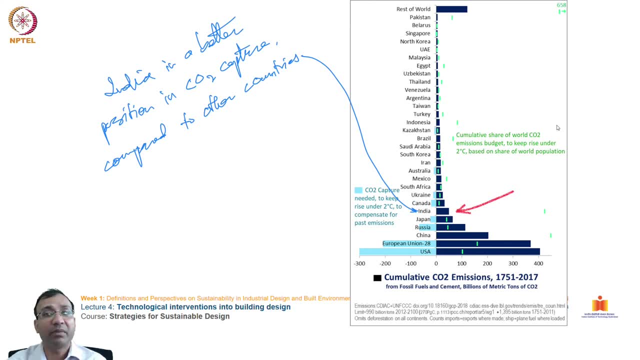 emission which has happened in these many years. okay, to bring it back to the normal where we can at the end of the year. we can bring it back to the normal where we can at the end of the year. we can at least go uh like under the two degrees, like a global warning, like temperature rise. so india for. 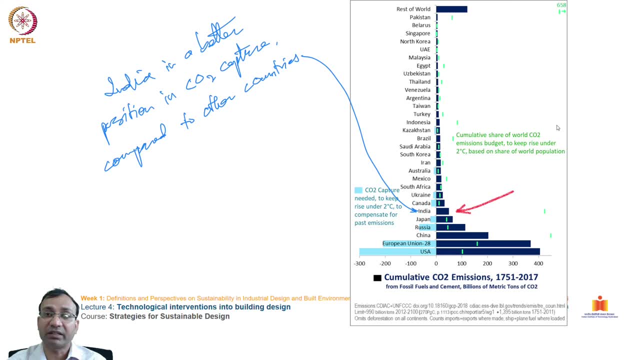 that it doesn't requires any, like you know, co2 capturing and this thing. that means we are not in a very deficit kind of situations. we are in a positive side. so india, as a like, a single like a country is, uh, is not doing that bad. i think it's doing fairly but, of course, in terms of like, 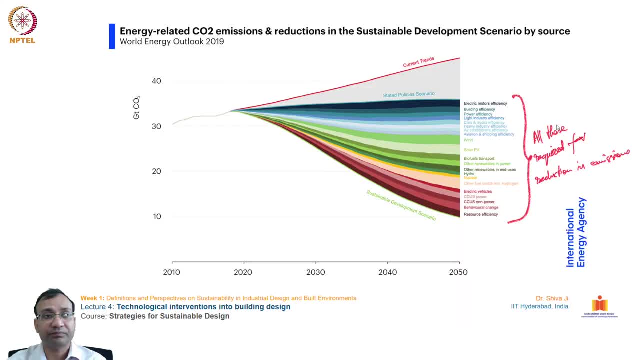 emissions. we should, we also need to control, and here on this slide you can see like what if that uh current trend of, uh like a rise in the co2, rise in the emission of the co2 it usually is- persist. so the the first line, the top line in the red, it suggests uh, the current. 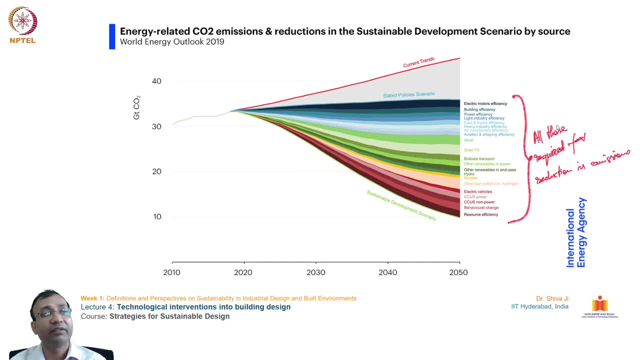 trend if the with the rate of this uh present actually emission, if it continues. so it's going to go like a way above. but there are some corrective measures which have been proposed by, like several agencies. okay, if we take them, so there are chances that this emission may come down. 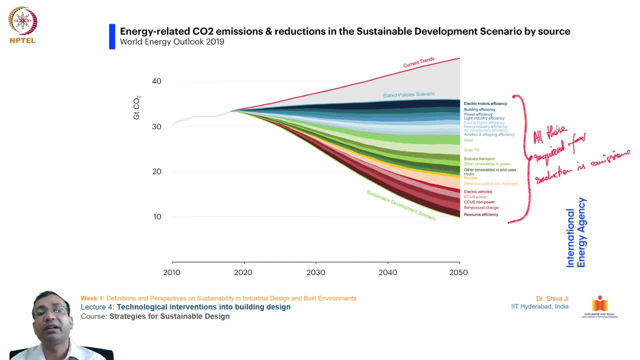 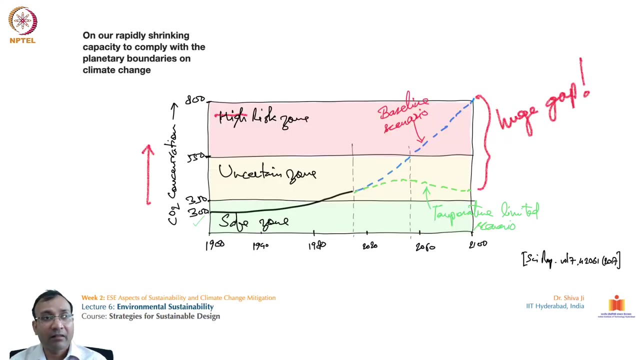 and there is one actually uh desired, like a sustainable development scenario also, which can be called if, thus, if this emission can be uh controlled, can be brought back uh to it's like a normal levels where it can envision, where the nature finds itself able to restore. okay, and here in this, uh, like a slide, you can understand, like, what are the like, uh, the the. 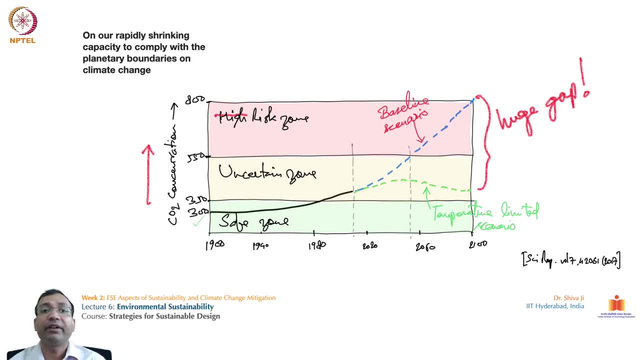 threshold from where, if there is like a uh way through which we can bring back that co2 emission levels to the normal, so it can still be considered at safe zone and where nature can restore and restore itself, uh. the second one is like the uncertain zone, where 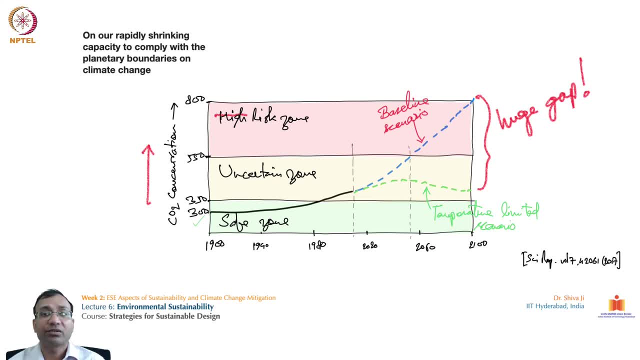 if the emission continues at the same pace so it can have some like a catastrophic effect. and the the third one is the very high uh high risk zone in in, in. if it the co2 emissions enter into that zone, then the uh resultant catastrophes could be like a very high 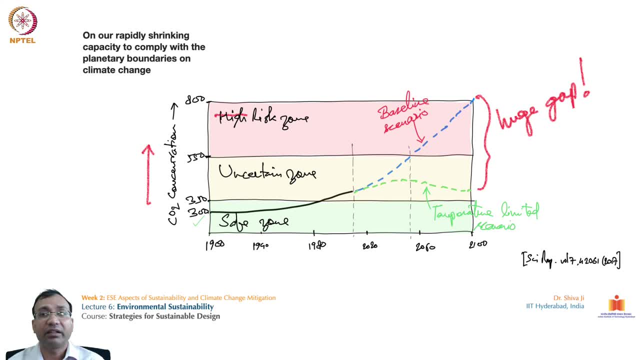 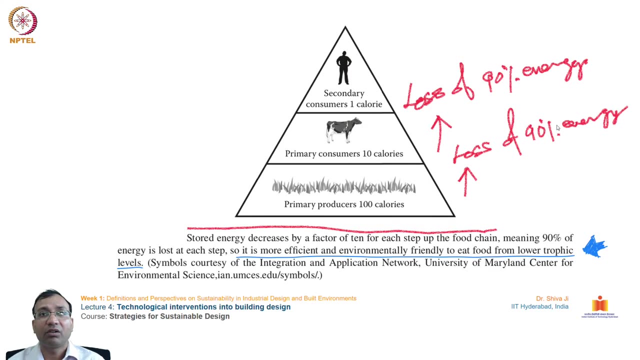 very, extremely bad, and that that's a very uh difficult actually to predict what could go wrong. so this phenomena can occur at the global level and there may be repercussions, like to be fit, like in the most of the countries, most of the places. uh, okay, so what to do? to like, uh, minimize the like energy consumption. minimize the consumption. 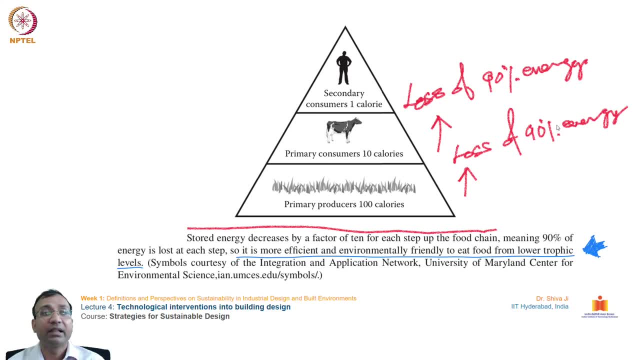 of resources. minimize this overall, like carbon footprint, is to understand. like what are our consumption habits are so the our consumption habits in the recent times have changed and a per person actually consumption of like resources has increased like manifold. so, as you can see in this pyramid, so the vegetables and uh vegetation based, actually plant-based fruit and trees based. 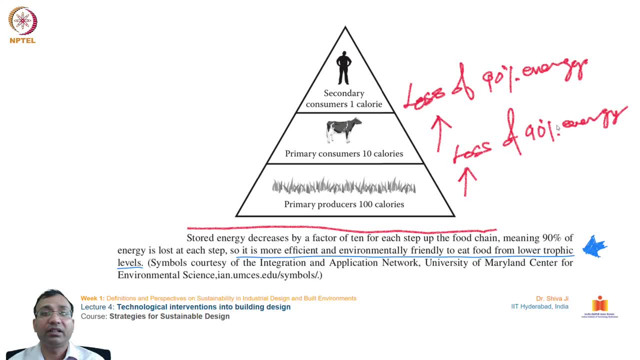 actually uh, these uh produce uh actually gives us like a hundred calories, if and then then at the next level, once the animals actually eat and the cattle actually consume, so there it reaches 10 percent of that and the 90 percent of that actually gets lost midway. and then the top level. 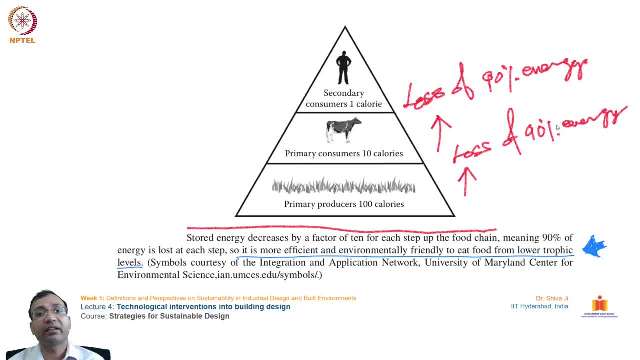 if you see it reaches by just one calorie. that means the further- like a 90 from the level two to three actually decreases. so we see there is actually trend of, like you know, the loss of energy at the rate of like 90 from one level to the next one. okay, so in order to actually, uh, save actually 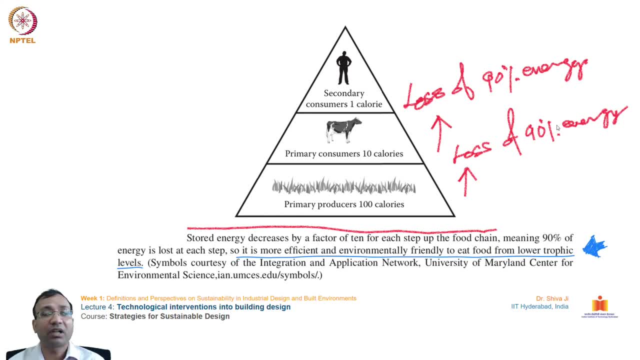 this overall like energy. okay, we need to come bring our like habits down to the lower actually base of the pyramid so that we can minimize the actually losses. so with this actually uh figure i would like to highlight over here, it is more efficient, environment friendly to eat food and consume actually resources from the 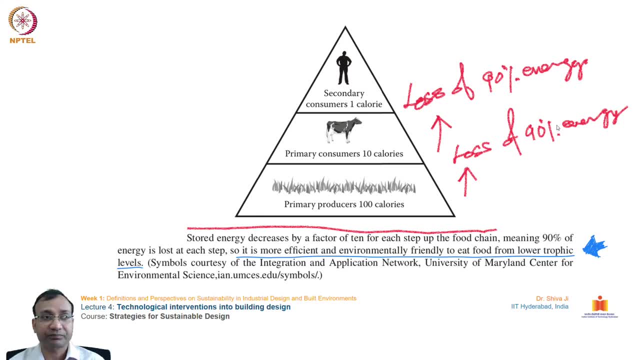 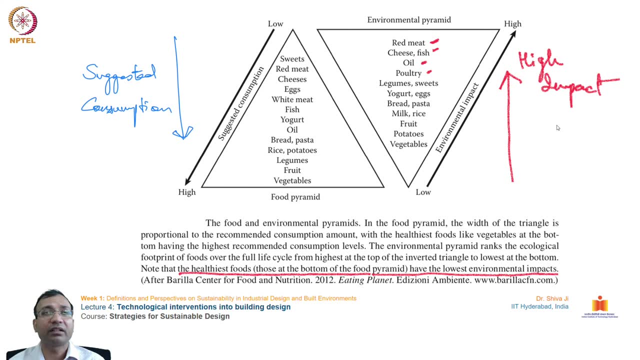 like a lower traffic, the lower strata of this pyramid. it is quite evident over here. with this slide you can see the. the common food items are actually listed down over here and they are arranged in two different orders: the the first. that pyramid on the left side suggests, like the suggested consumption from low to high. 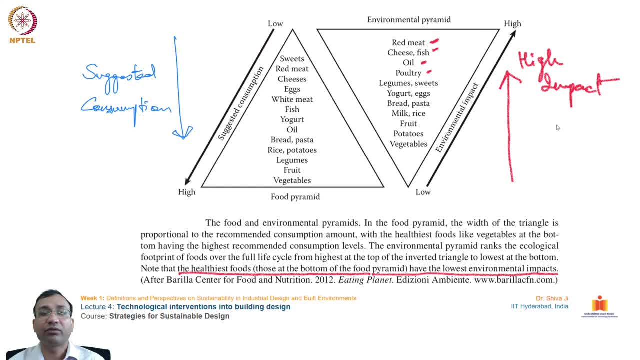 uh, in in terms of like in this pyramid. so the vegetables, fruit, legumes- they come at the bottom of this, and the sweets, red meat, cheese, eggs, white meat, etc. they come at the top of this. actually, okay, and in terms of like, a environmental impact of them. so the first one talks about the energy. 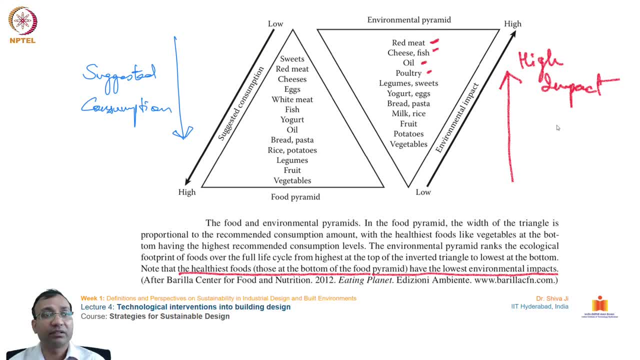 the second one talks about the impact. okay, so the- this actually we can see this actually pyramid gets inverted. the impact of the, the, the top most item which is there in the food chain, has the suggest like a directly that we should actually go for a uh diet which is like a vegetable based.